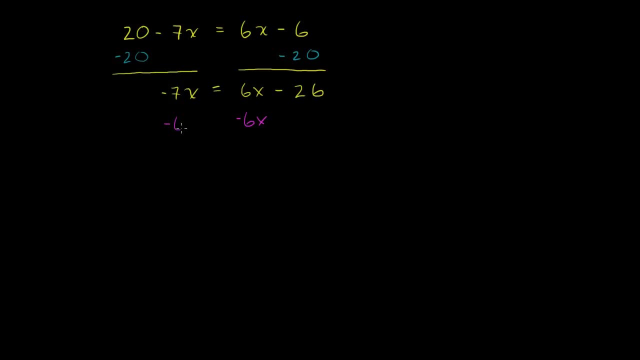 So let's subtract 6x from the right, Subtract 6x from the left, And what do we get? What do we get? The left-hand side- negative 7x minus 6x. That's negative 13x. 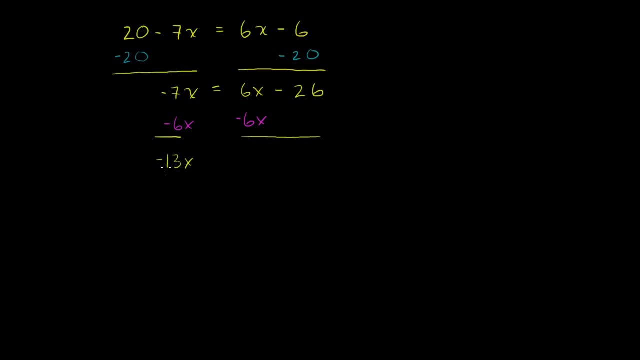 Right, Negative 7 of something minus another 6 of that something is going to be negative 13 of that something And that is going to be equal to 6x minus 6x. That cancels out. That was the whole point behind subtracting negative 6x. 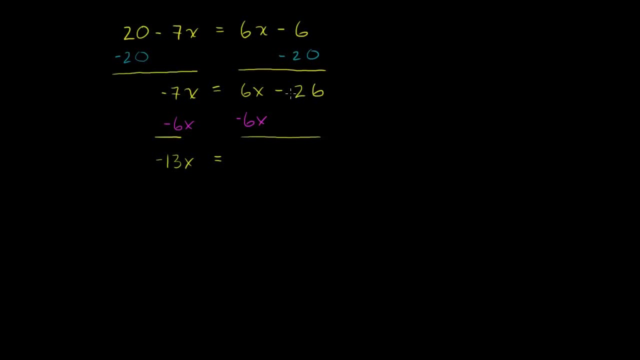 That was the whole point behind subtracting negative 6x, And then we have just a negative 26 or minus 26,, depending on how you want to view it. So just negative 13x is equal to negative 26.. Now our whole goal, just to remember. 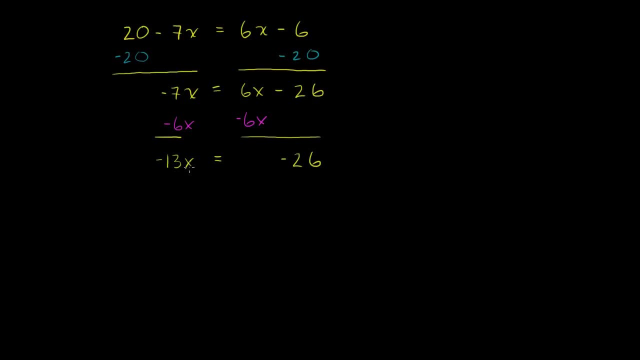 is to isolate the x, And we have a negative 13 times the x here. So the best way to isolate it is if we have something times x. if we divide by that something, we'll isolate the x. So let's divide by negative 13.. 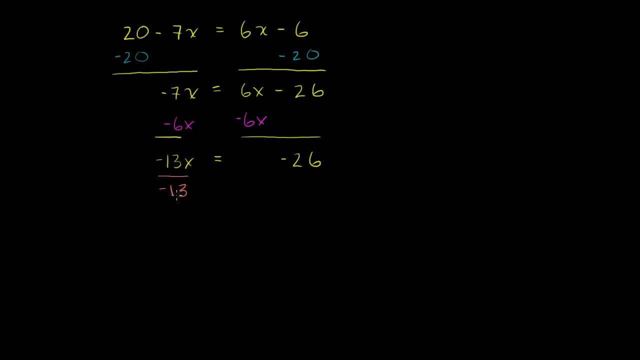 Now You know by now, anything you do to the left-hand side of an equation you have to do to the right-hand side. So we're going to have to divide both sides of the equation by negative 13.. Now what does the left-hand side become? 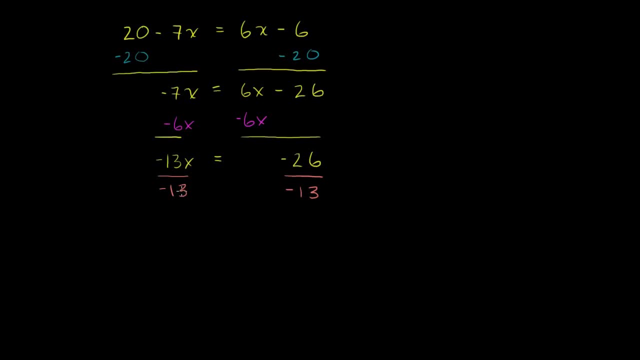 Negative 13 times x divided by negative 13.. That's just going to be x. You multiply something times x divided by the something. you're just going to be left with an x, So the left-hand side just becomes an x. x is equal to negative 26 divided by negative 13.. 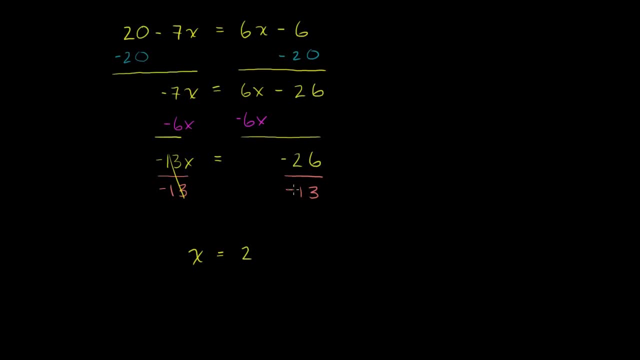 Well, that's just positive: 2.. A negative divided by a negative is a positive. 26 divided by 13 is 2.. And that is our answer. Now let's verify that it really works. That's the fun thing about algebra. 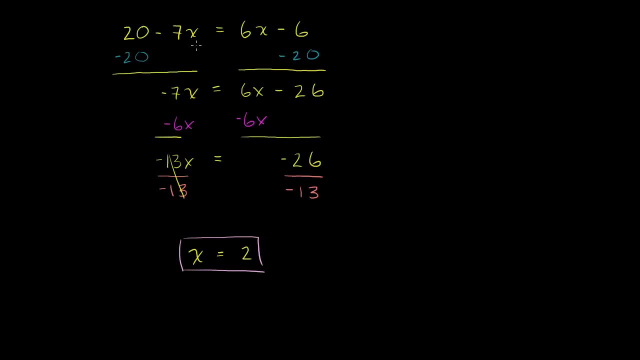 You can always make sure that you got the right answer, So let's substitute it back into the original equation. So we have 20 minus 7 times x. x is 2.. Is equal to 6 times x. We've solved for x.